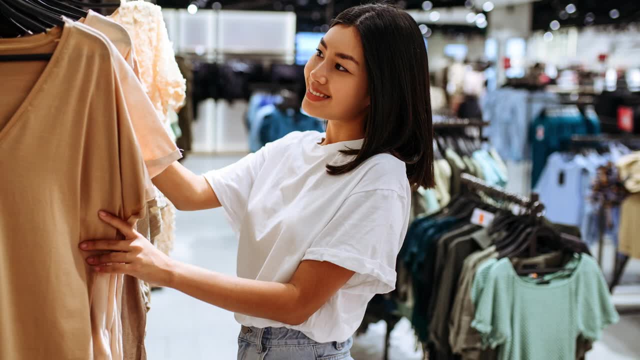 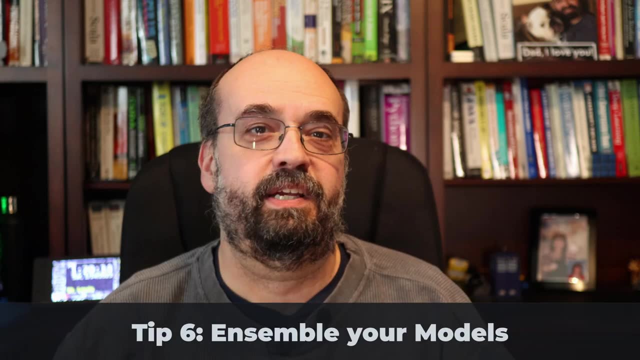 no one-size-fits-all solution when it comes to machine learning, so experiment with different algorithms and models to find the one that works best for your problem. Tip six: use insoluble techniques. Ensembling is a powerful technique that combines the predictions of multiple models. 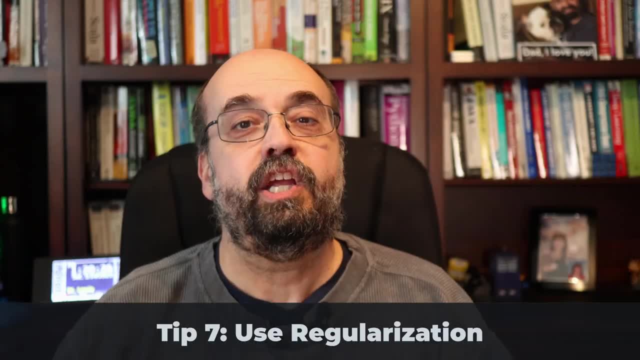 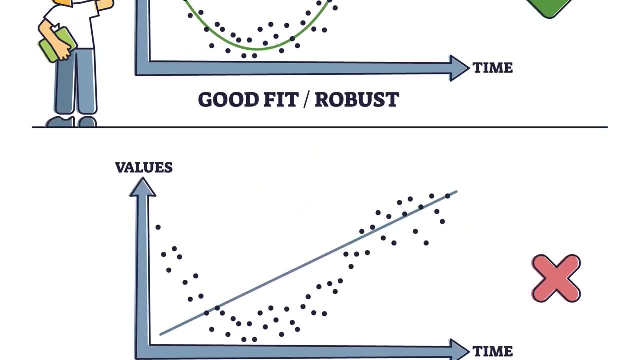 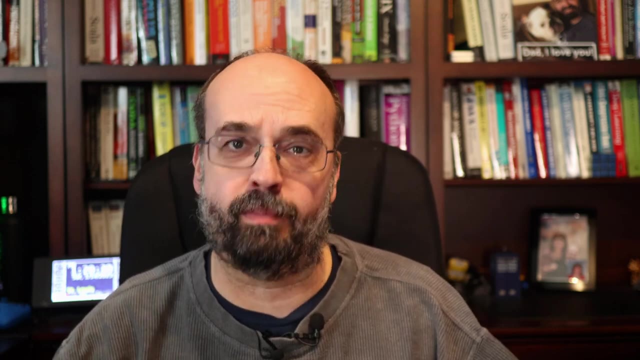 to achieve better results. Tip seven: use regularization to prevent overfitting. Overfitting occurs when a model is too complex and memorizes the training data instead of generalizing to new examples. Regularization is a technique that helps prevent this by adding a penalty term. 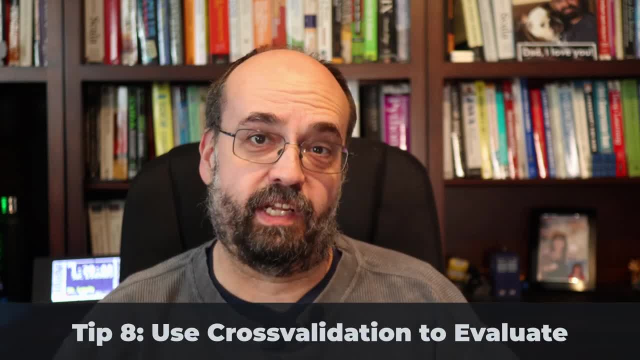 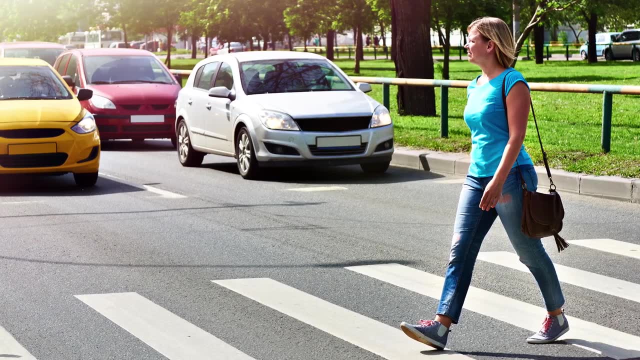 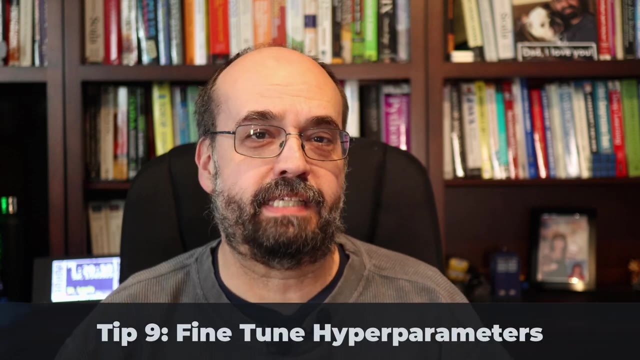 to the model's complexity. Tip eight: use cross-validation to evaluate your model. Cross-validation is a technique that allows you to evaluate your model on different subsets of the data, which helps you to reduce the risk of overfitting. Tip nine: fine-tune your model's. 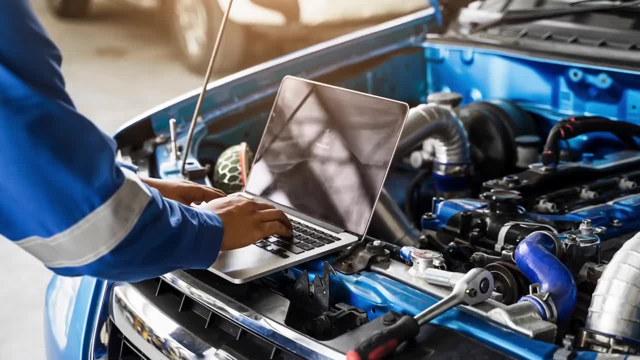 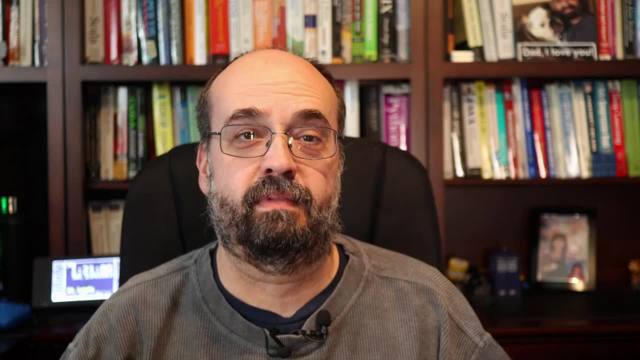 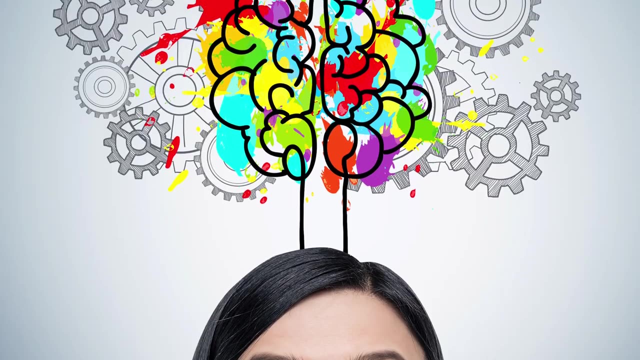 hyperparameters. Hyperparameters are the parameters that control the behavior of a machine learning model. Fine-tuning them can have a big impact on model performance. Tip 10,: keep an open mind and be willing to experiment. Machine learning is an iterative process and it's important to be. 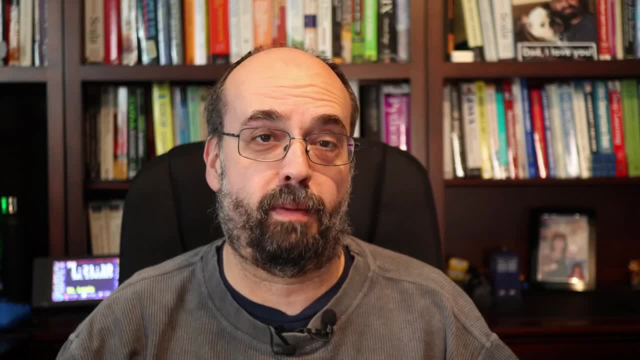 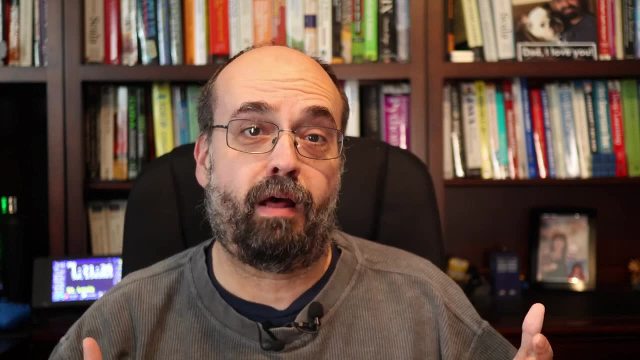 open to new ideas and willing to experiment with different approaches. So these are our 10 tips for improving the accuracy of your model. We hope you found them helpful and we wish you the best of luck in your machine learning journey. Thanks for watching. Okay, guess what This was actually? 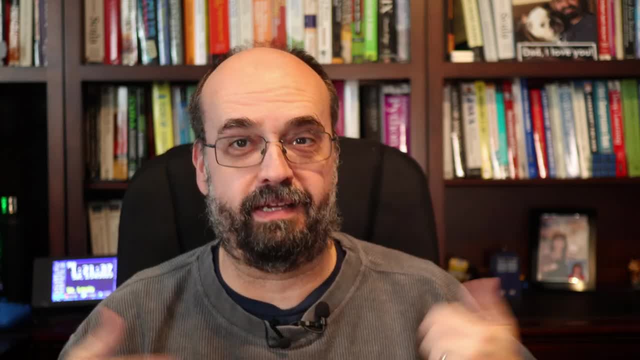 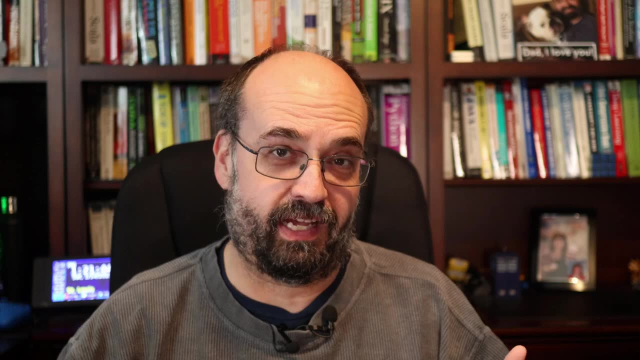 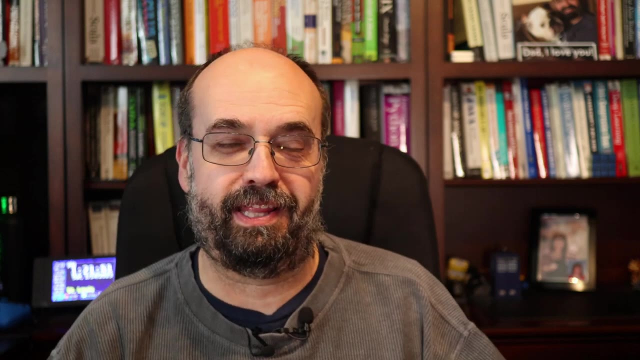 a video completed entirely, except for the narrator here from ChatGPT. I let ChatGPT pick the title of the video that we were going to produce. I let it write the description that you saw in YouTube. got advice on the thumbnail. 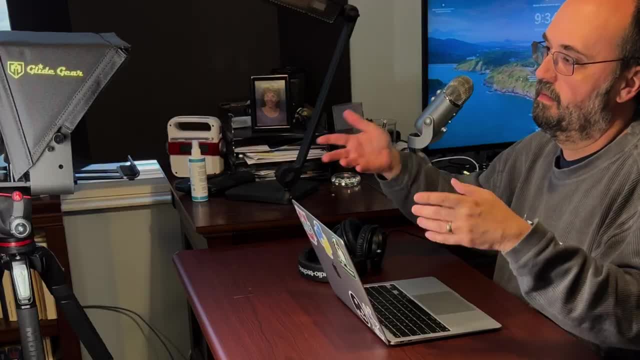 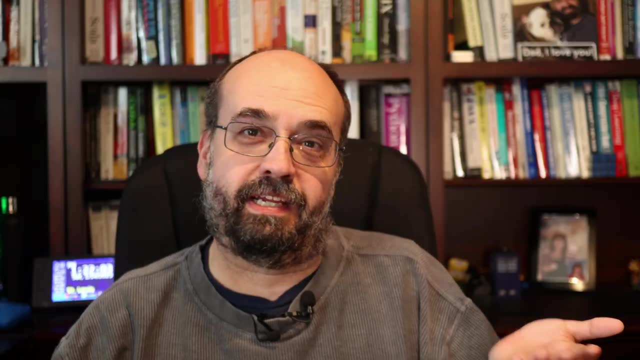 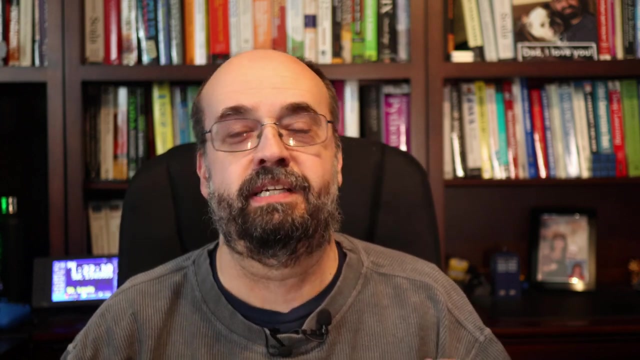 and then had it script the entire thing. So I am sitting here actually in front of a teleprompter just reading the script that ChatGPT wrote for me. What do you think? If you like it better than my other videos, I guess I'm done and I welcome my ChatGPT overlords. If not, 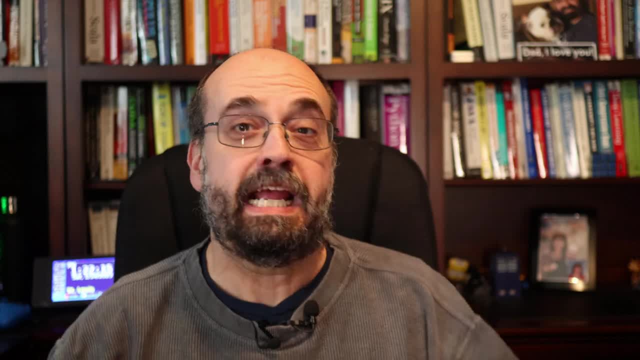 But, oh, but you know, the thing that it forgot to say is: smash the like button and subscribe if you found this video helpful. Thank you very much.